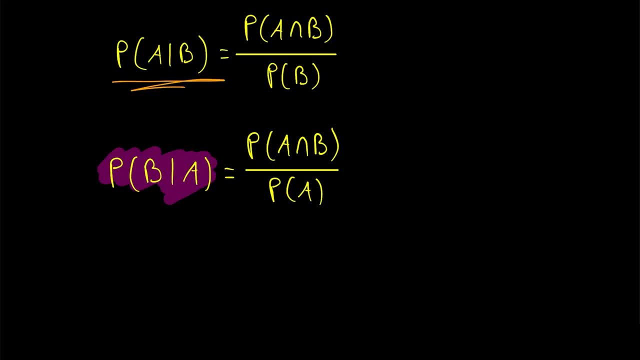 whereas we do know the other one, or at the very least it's easy to compute. Bayes' theorem helps us in this situation. We can write the probability of A given B or calculate the probability of A given B in terms of the probability of B given A. 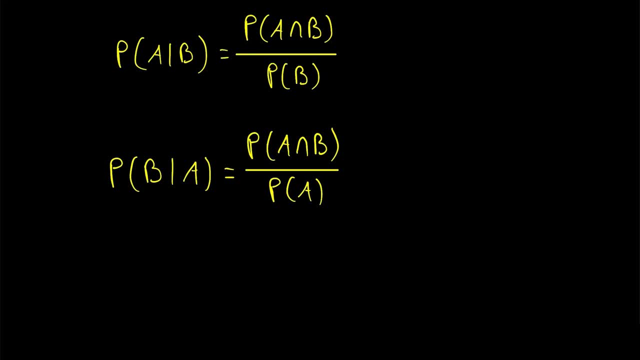 And we can just use these two simple definitions to do that. Notice that the probability of A intersect B is in both of these expressions Here, with the probability of B given A. if we multiply both sides of the equation by the probability of A, we will have the probability of A intersect B in terms of. 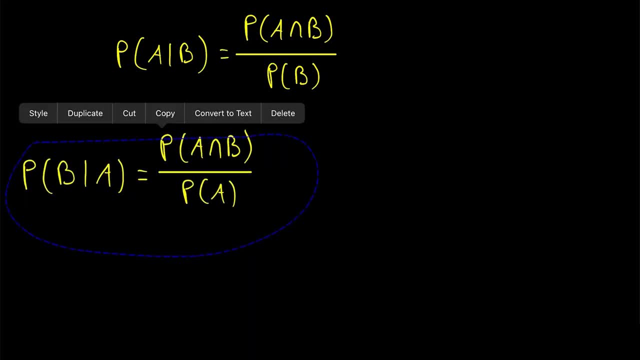 this conditional probability. So let's just do that real quick Again. just multiply both sides of the equation by the probability of A, And that gives us that the probability of A intersect B is equal to the probability of B given A multiplied by the probability of A. 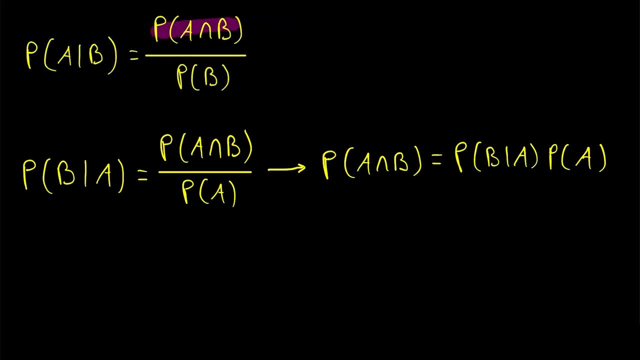 And now check this out. We've got this nice expression for the probability of A intersect B, So let's do some substitution. We have that the probability of A given B is equal to the probability of A intersect B, which is equal to this, So we can just do a little bit of copy-paste. 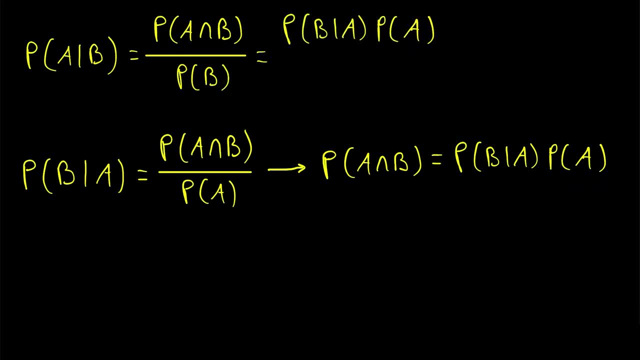 here, That's our numerator by substitution, And then in the denominator we still just have the probability of B. Now just getting rid of this middle part of the equality and changing the color to make this stand out. this, my friends, is Bayes' theorem. 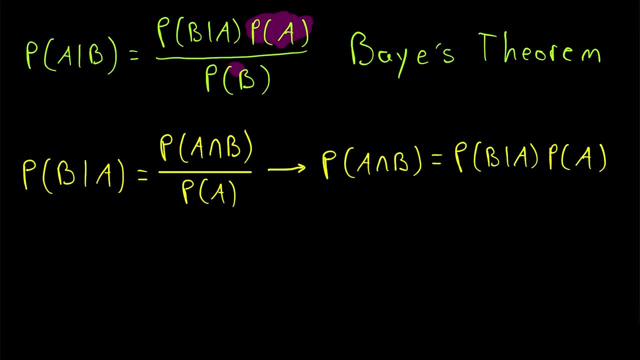 So Bayes' theorem tells us, if we know the probability of A and the probability of B and we know how A occurring affects the probability of B occurring, if we know all of this, then we can calculate the conditional probability of A given B. And this theorem really is. 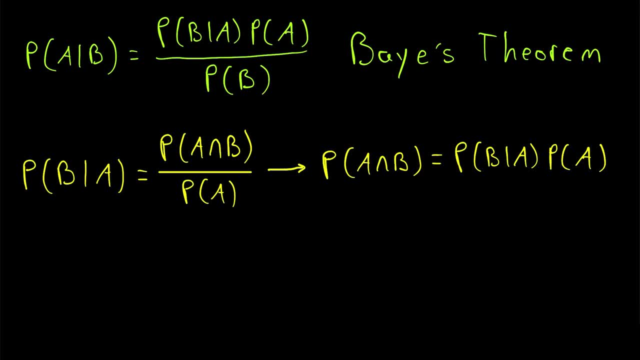 brilliant in its simplicity and in its usefulness And I really want to draw attention to the fact here. Notice, we are calculating the probability of A given B using the reverse conditional probability, the probability of B given A. It's pretty sweet And, of course, 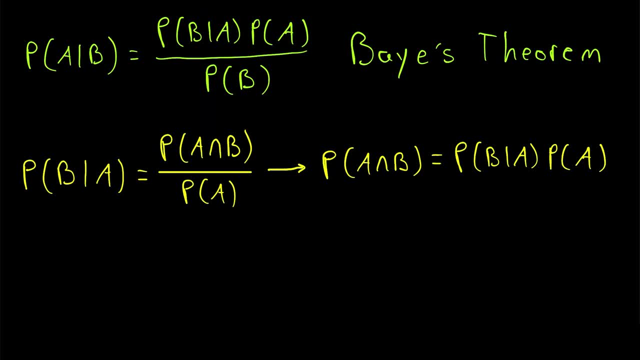 we were able to arrive at this theorem pretty easily, So it's not really necessary to memorize it, but a lot of you will probably be using it so much that you're going to end up memorizing it pretty quickly. anyways, The way I always remember Bayes' theorem is that I know it's an 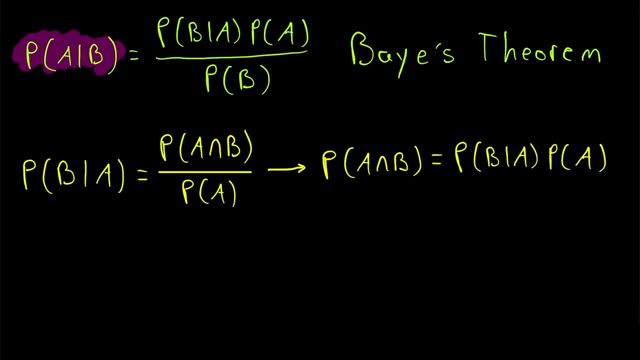 expression for conditional probability. So it starts with the probability of A given B, And I know that it lets us write that probability in terms of the reverse conditional, the probability of B given A. And then I know, since A comes first, we've got probability of A in the numerator. 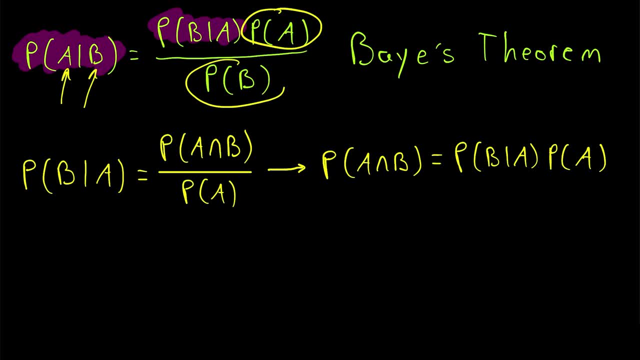 And since B comes second on the left-hand side we've got probability of B in the denominator. The A given B in the conditional probability on the left is kind of reminiscent of probability of A divided by the probability of B. So that's just. 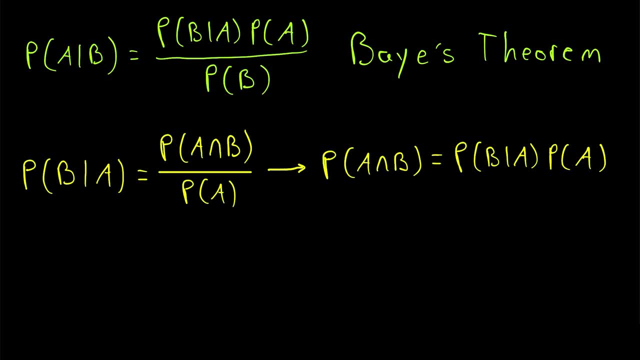 how I remember it. We'll get to an example of applying the theorem in just a minute, But first I want to mention doing the calculations with. this. theorem is not always quite as simple as this appears Oftentimes. instead of just knowing the probability of B, the sample space will be. 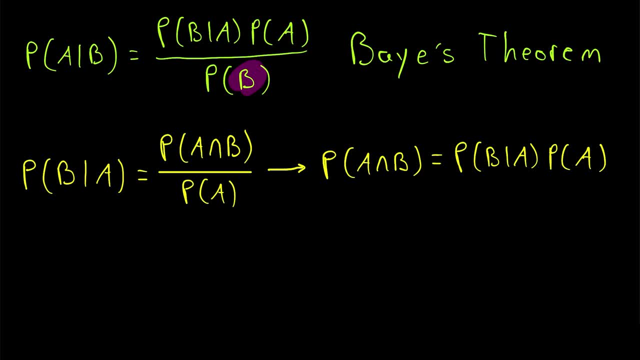 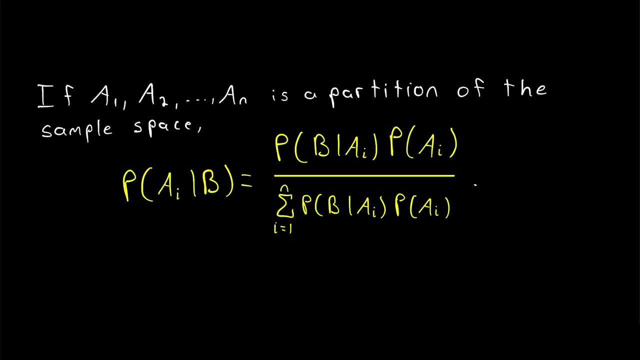 partitioned into a bunch of different events, And so we'll have to calculate the probability of B using the law of total probability, which isn't a huge difficulty, but it's something to keep in mind. So let's check this statement real quick, so we know. 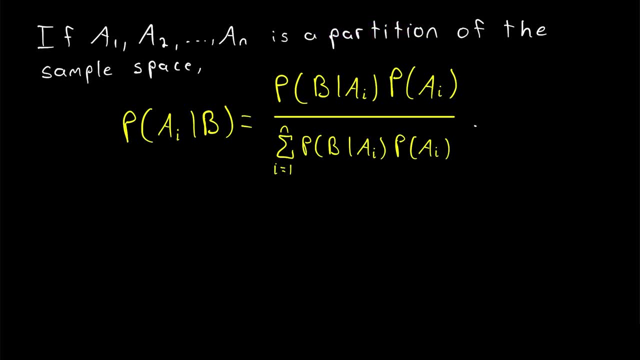 If our sample space has been partitioned into n sets, A1, A2, and so on up through A- n, then we can write Bayes' theorem like this: The probability of a particular A i occurring, given that B has occurred, is equal to the same sort of numerator that we saw before the probability of B. 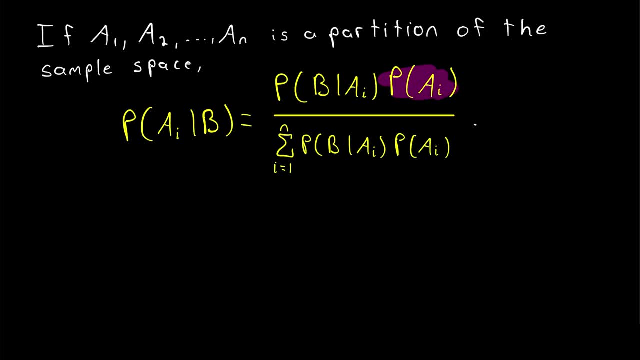 given that A i has occurred, multiplied by the probability of A i occurring, divided by the probability of B- And this is where we use our law of total probability of B. So if we have a probability with the partitions of the sample space, we're just adding up all the weighted. 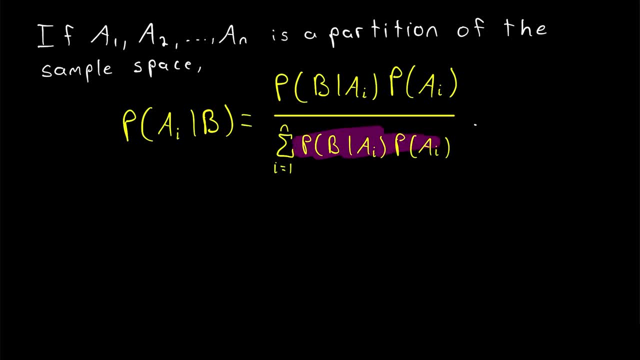 conditional probabilities of B occurring in the different partitions of the sample space. If you want a recap on the law of total probability, I'll leave a link in the description to a lesson I did on that as well. Now let's just go ahead and get into a fun little example problem. 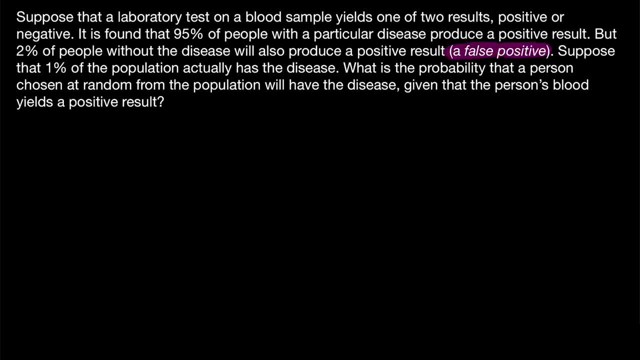 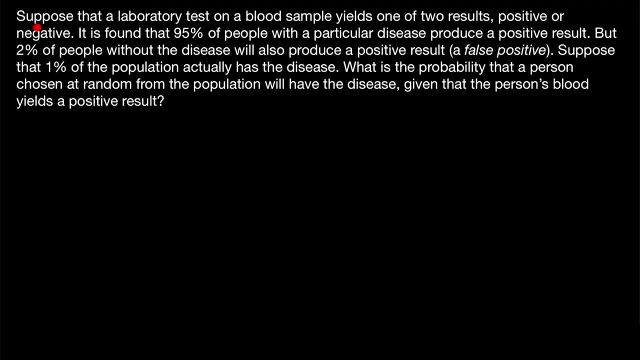 This is a problem about false positives, which I think is a great way to introduce Bayes' theorem. It shows us how the theorem can really give us some useful and at times surprising results. Suppose that a laboratory test on a blood sample yields one of two results. 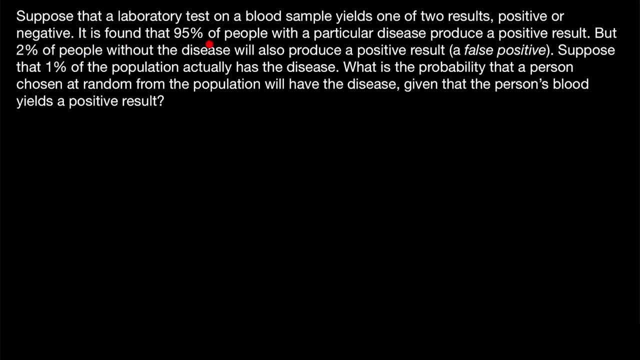 positive or negative. It's found that 95% of people with a particular disease produce a positive result, but 2% of people without the disease also produce a positive result, thus called a false positive. since it's a positive result, that isn't correct Suppose. 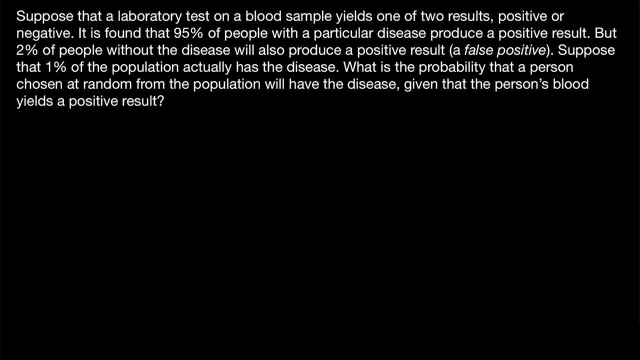 that 1% of the population actually has the disease, then what's the probability that a person chosen at random from the population will have the disease, given that the person's blood yields a positive result? And notice that this is certainly an important question If you test. 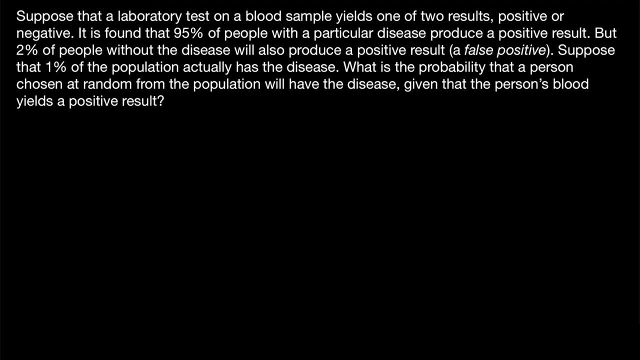 positive for a disease, a lot of people might think immediately that means they have the disease, but of course there is a sort of probability attached to it, and that's a probability that you would want to know. What's the probability that it's actually accurate, given that I've 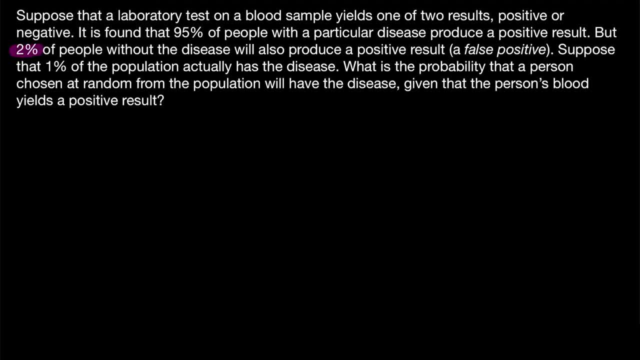 tested positive. You might think reasonably that since very few people without the disease produce a positive result and pretty much everybody with the disease produces a positive result, that if you had a positive result you probably have the disease. But as we'll see, 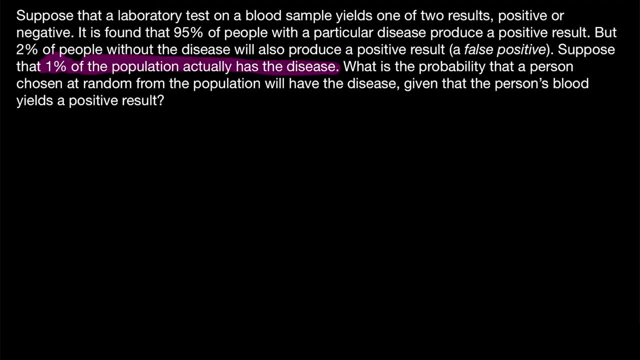 the amount of people who actually have the disease is so small that if you do test positive, there's a surprisingly large chance that that test is inaccurate. So let's see what the actual numbers are by using Bayes' theorem. For starters, let's just write the probabilities that we know. 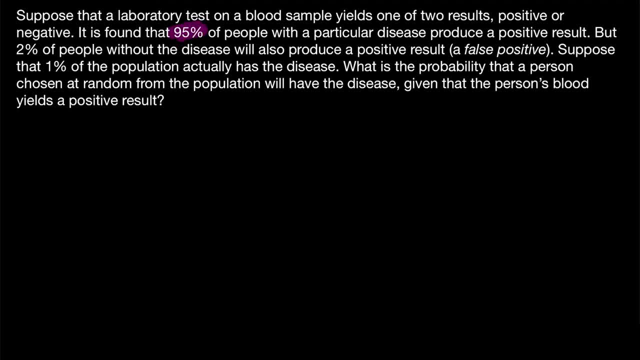 We've got that. it's found that 95% of people with a particular disease produce a positive result. So what is that? Well, that means if we know someone has the disease, there's a 95% chance they'll produce a positive result. So we could say: 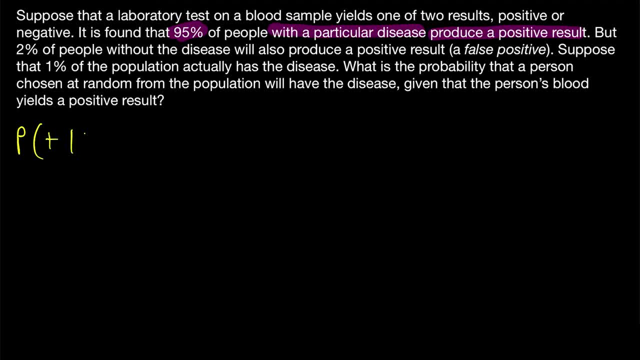 the probability of a positive result, given that someone has the disease. so probability of positive, given D is equal to 95% or 0.95.. Then we have that 2% of people without the disease also produce a positive result. So what is that? Well, that means if we know someone has the disease, there's a 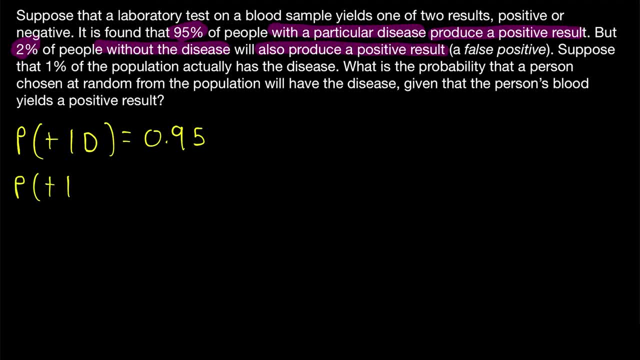 So this tells us that there's a probability of a positive result for people who don't have the disease, So we'll write the negation of D: don't have the disease. This is equal to 2% or 0.02.. 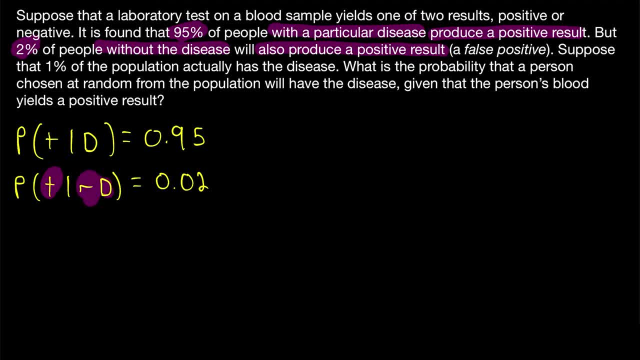 The probability of testing positive, given that someone doesn't have the disease, is 2%. Lastly, we have that 1% of the population actually has the disease. So this is our probability of D. The probability of having the disease is 1% or 0.01.. 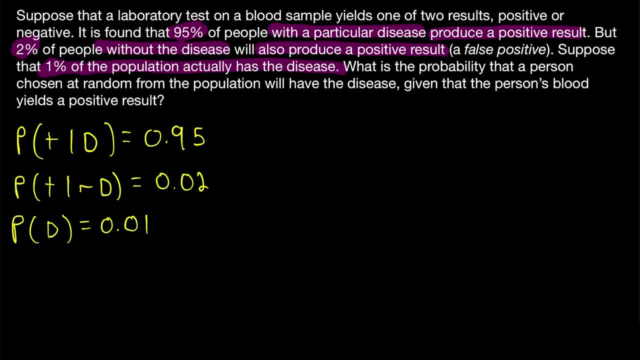 All right now. what are we actually trying to find? Well, we want to know the probability that a person chosen at random from the population will have the disease, given that their blood yielded a positive result. So what we want to know is: what's the probability of actually having the? 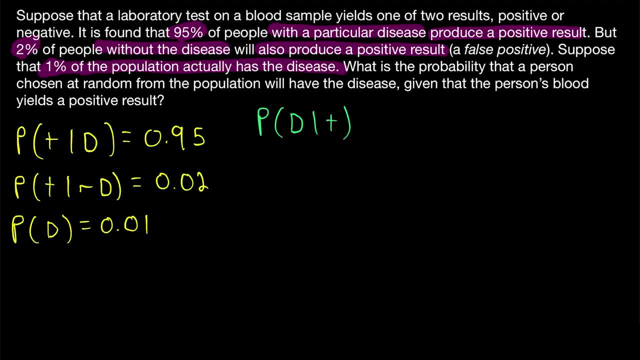 disease given a positive result. Of course, it's not obvious what this probability should be, but we already know the other conditional probability, the probability of a positive result given that someone has the disease. We know that's 95%, So let's go ahead and try using Bayes' theorem to solve the problem. 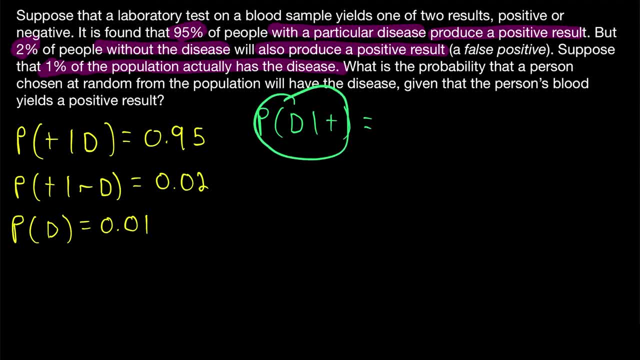 Recall that Bayes' theorem tells us how to calculate a conditional probability using the conditional probability in the other order. So in the numerator we have the probability of a positive result, given that someone has the disease, multiplied by the probability of actually having the disease. 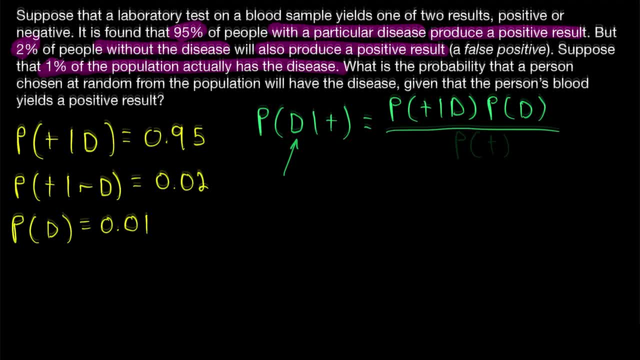 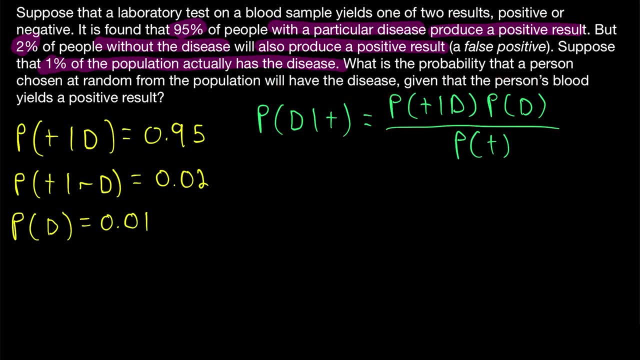 divided by the probability of a positive test. All right, so will we be able to use this to calculate the probability of a positive test? Well, we're going to have to find out how to do that. Our conditional probability. Well, we know what the probability of a positive result. 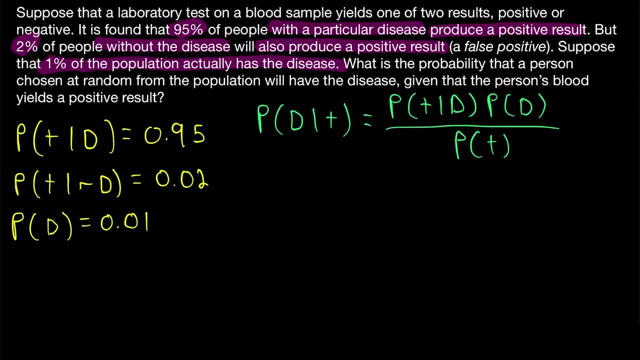 given that someone has the disease is, We know what the probability of having the disease is. We're not directly given the probability of a positive result, but someone either has the disease or they don't, So we can calculate the probability of a positive result using these. 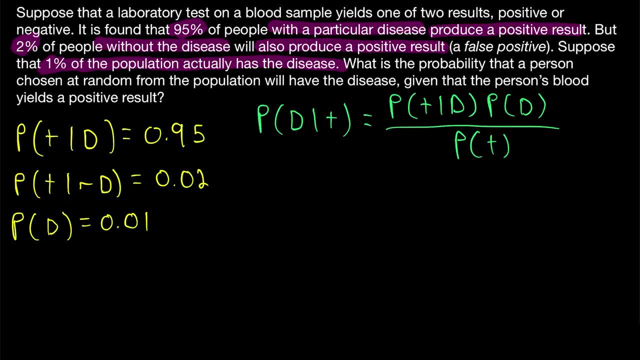 two probabilities and the law of total probability. So let's get cracking. We'll start writing the expression over here, just so we've got some more room to write it. The probability of a positive result, given that someone has the disease we know, is 0.95.. So we've got 0.95. 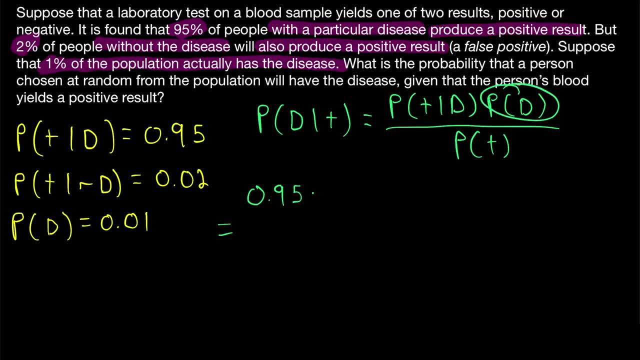 multiplied by what? The probability that someone has the disease, which we know, is 0.01.. So multiplied by 0.01, and then we've just got our denominator to worry about. I'm going to make this fraction bar nice and big, so we've got plenty of room to write it In the denominator. we just need. 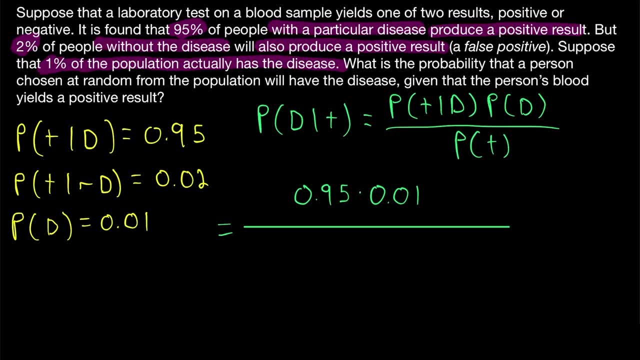 to calculate the probability of a positive result. Here's where we use our law of total probability. we know that the probability of a positive result, given that someone has the disease, is 0.95.. Now, of course, we should weight that by the probability of someone actually having. 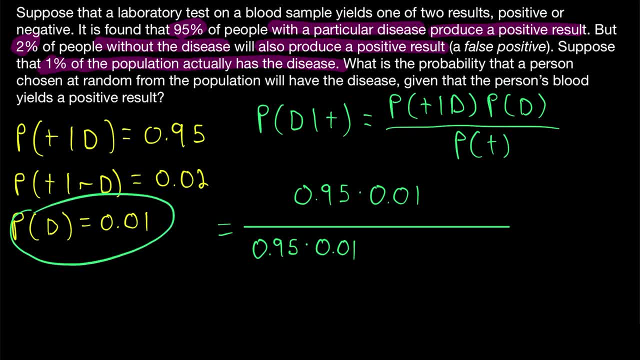 the disease, which is 0.01.. We were given that, And then the only other possibility is that someone doesn't have the disease. In that case, the probability of a positive result is 2% or 0.02.. And of course we should weight that by the probability of someone not having the disease. 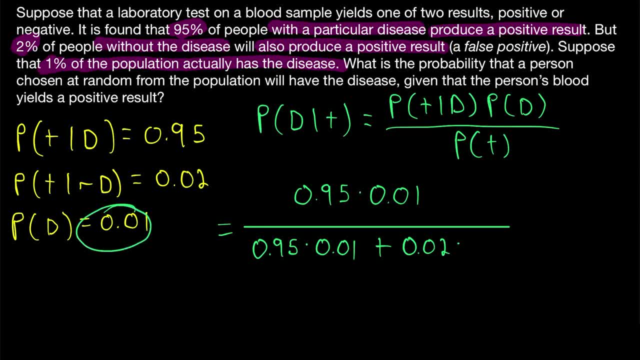 If the probability of having the disease is 0.01,, then of course, the probability of not having the disease is 0.99.. And this, my friends, is approximately 0.32, or 32%. So how about that? 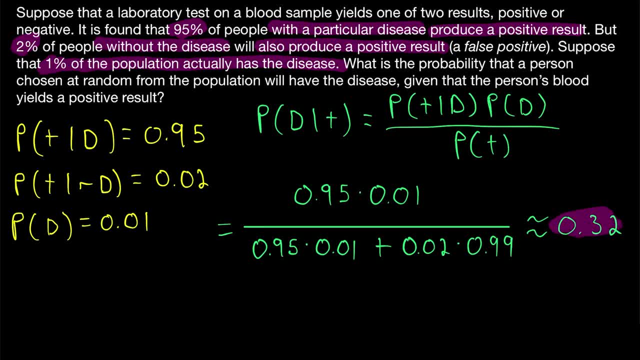 Remember what this actually is. This tells us that if we test positive, the probability that we have the disease, given that positive result, is only a meager 32%. So even if we test positive for this disease, we're not going to get 0.02.. So we're going to get 0.02.. So if we test positive for this, 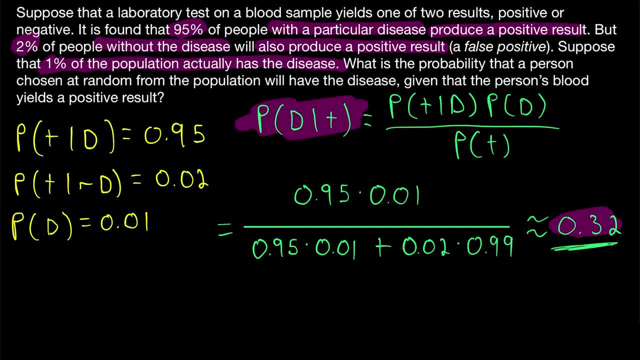 it's more likely than not that we don't have it. Amazing, and that's the power of Bayes' theorem. There's, of course, plenty more we could say about the theorem and plenty more examples we could go over, and we'll do more of that in future lessons. 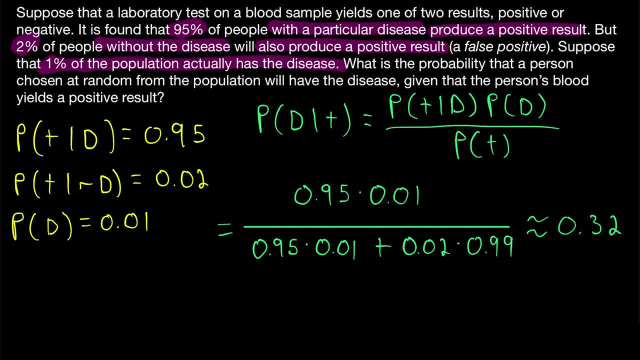 And be sure to let me know if there are any particular types of Bayes' theorem problems you'd like to see a lesson on in the future, and I'll try to get to that sooner than later. In any event, I hope this video helped you understand what Bayes' theorem is and how to use it. 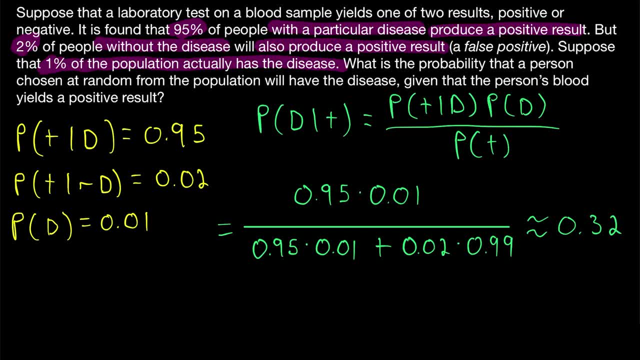 Let me know in the comments if you got any questions, need anything clarified or have any other video requests. If you'd like to help support the channel, I'd really appreciate a small donation on PayPal or a small monthly pledge on Patreon. Links to both of those are in the description. 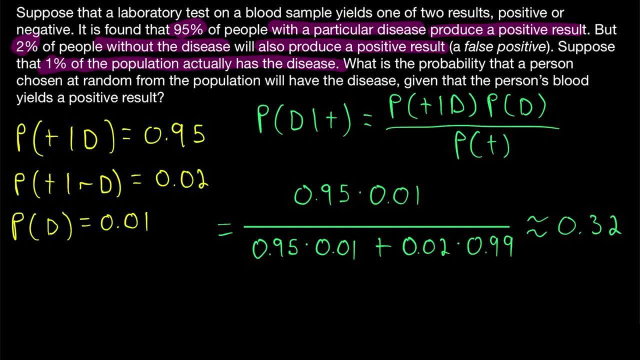 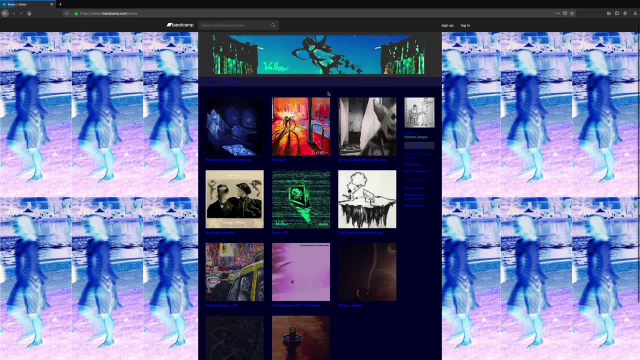 Thank you very much for watching. I'll see you next time and be sure to subscribe for the swankiest math lessons on the internet. And a big thanks to Valo who, upon my request, kindly gave me permission to use his music in my math lessons. 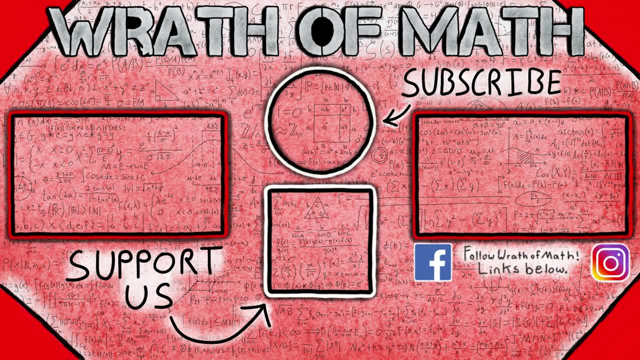 Links to his music in the description. Keep tomorrow on your wings. But everyone else just looks at you and sighs: I'd like to live, But I'm too shy.